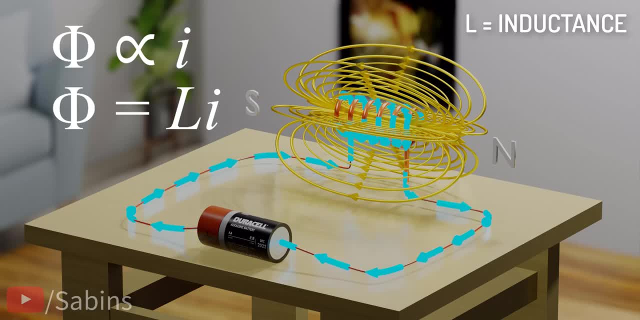 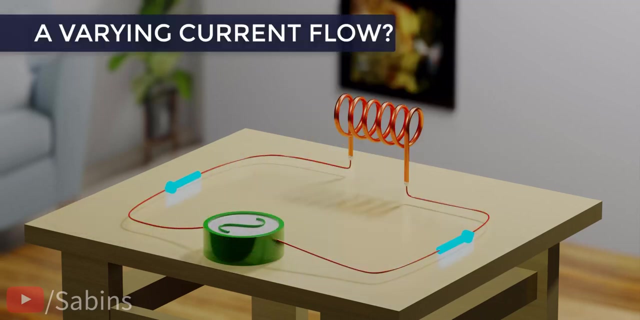 A constant called inductance connects between the magnetic flux and the current's value. The value of inductance depends purely on the geometry of the coil. Now for the most important part of this video: What will happen if the current through the coil changes? 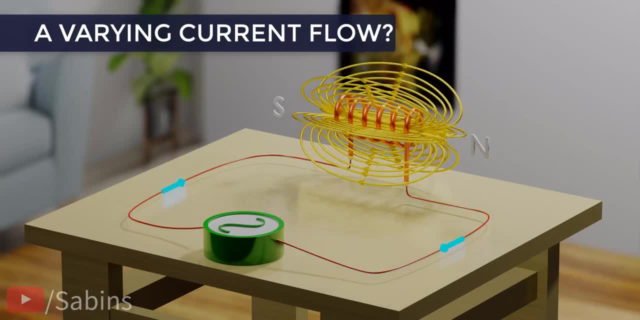 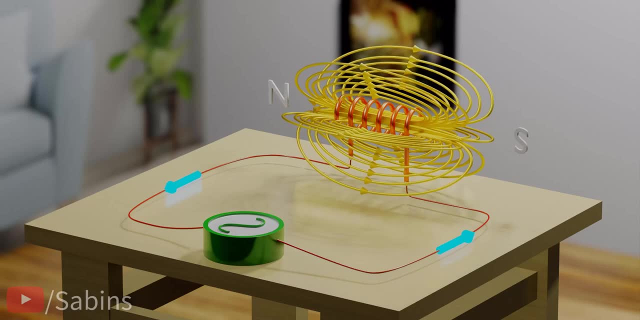 When the current changes, the magnetic flux that the coil produces also changes, Which means we need to study the effect of this varying magnetic flux on the coil. To study the effect of varying magnetic flux on a coil, we need to introduce Faraday's law. 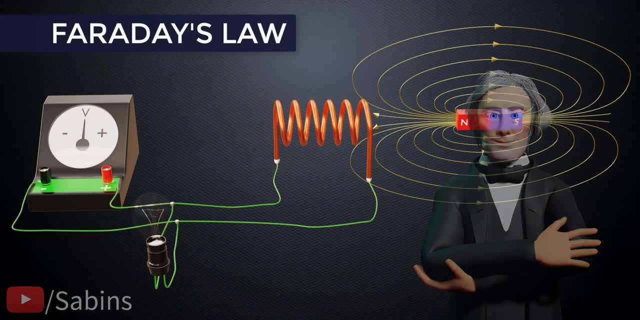 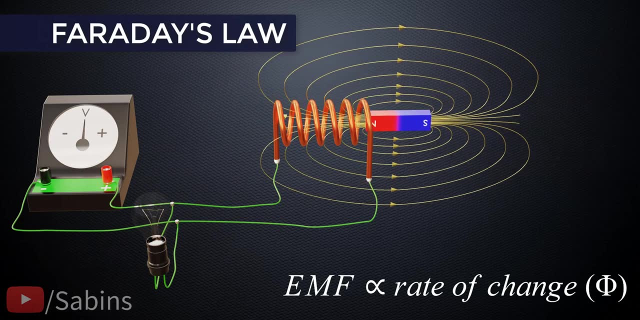 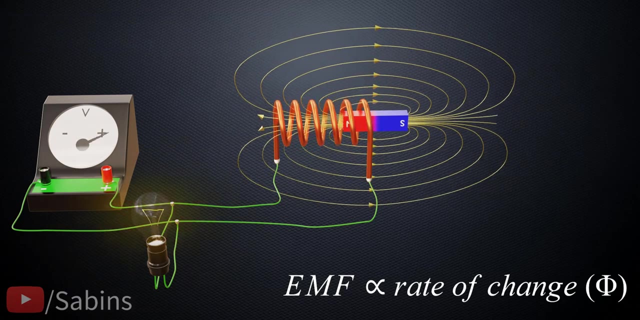 The great scientist Michael Faraday said: if the magnetic flux changes across a loop, it will induce an EMF across it. Here you can see that the permanent magnet approaches or leaves the loop, It will induce an EMF across it. This result occurs because the movement of the permanent magnet causes a varying magnetic flux on the loop. 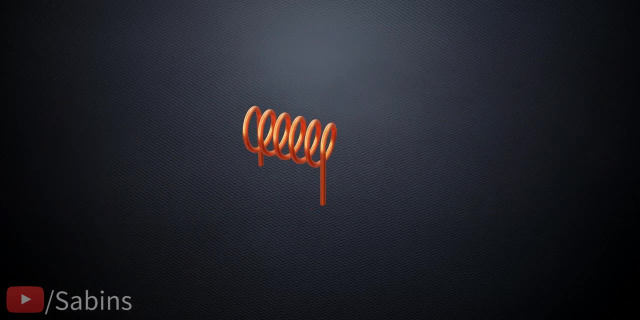 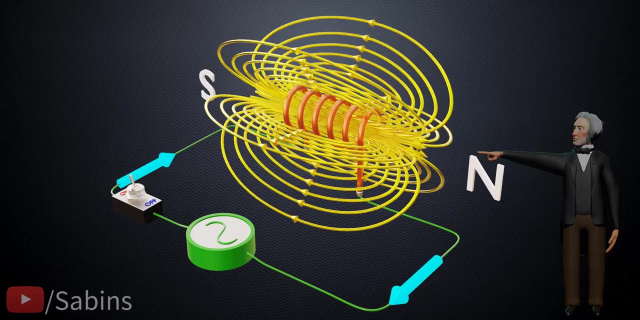 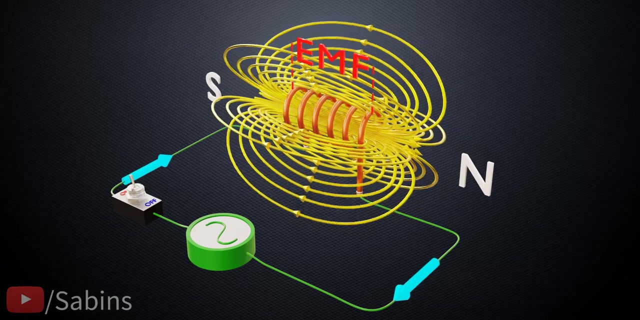 Now let's apply Faraday's law to an inductor connected across an AC power supply. According to Faraday's law, the varying magnetic flux that the AC power source produces will definitely produce an EMF across it. This EMF is known as back EMF and this phenomenon is called self-induction. 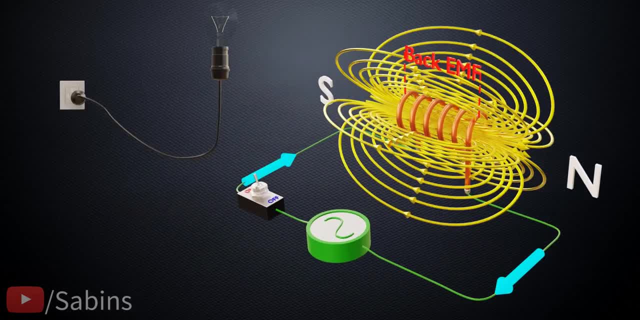 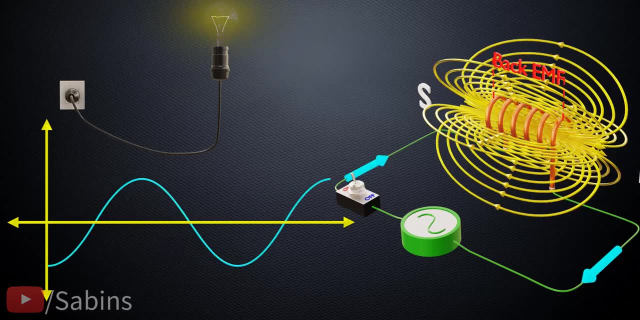 The electricity we use everywhere is sinusoidal in nature. It's therefore very important to study the effect of a sinusoidally varying EMF across the inductor. You might have noted that in Faraday's law, everything is about the rate of change. 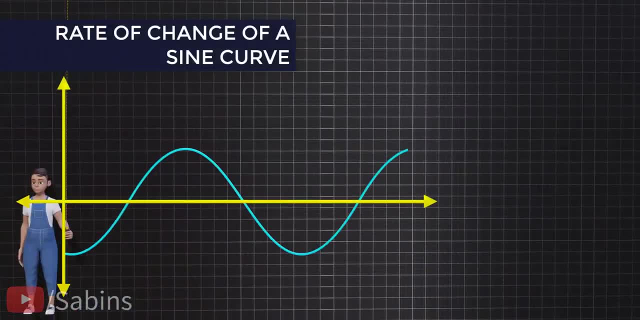 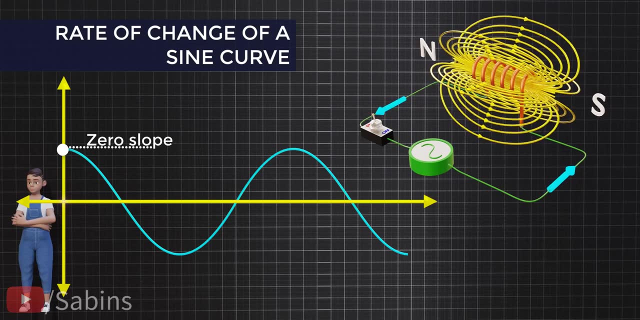 So let's study more about a sine curve's rate of change. Clearly, for the sine curve, the change is zero when the current is at the peak and the change is maximal when the current is zero. This is one interesting property of a sine curve. 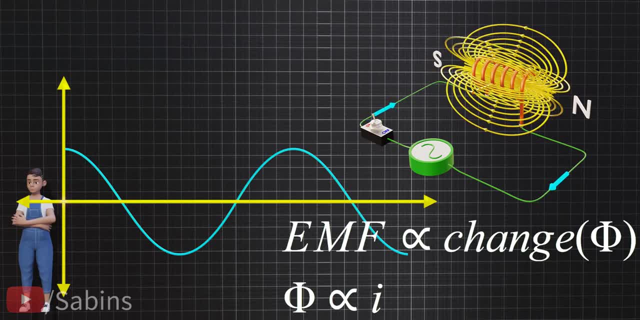 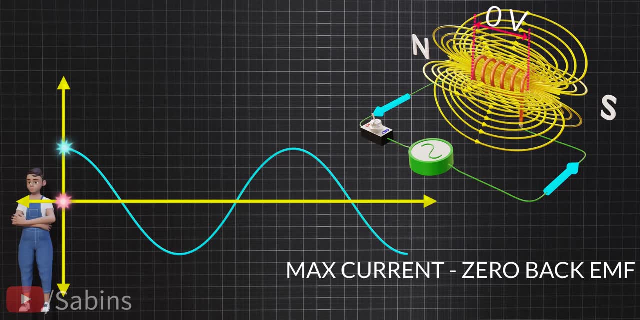 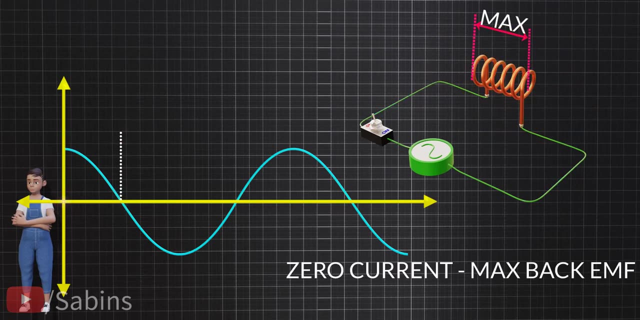 The EMF it induces is proportional to the change in current. Therefore, the EMF across the inductor is zero when the current is at maximum and the EMF is at maximum when the current is zero. In short, the back EMF will vary as shown.